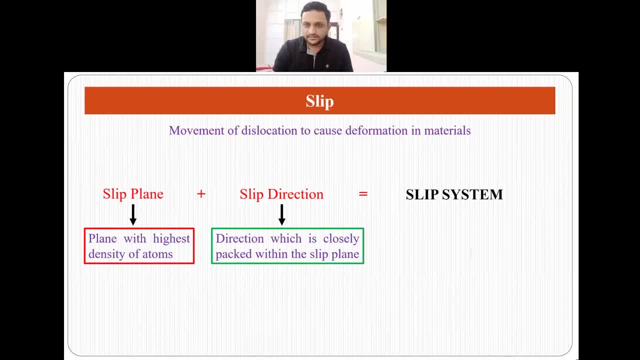 It means the dislocations or how the dislocations are moving. And since these dislocations are moving, it will lead to plastic deformation in materials, and that is why we can define slip as movement of dislocation to cause deformation in materials. Now this slip has two components. 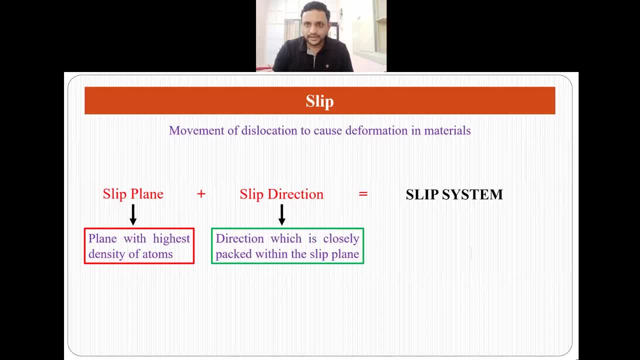 slip plane and slip direction. Slip plane is a plane with highest density of atoms and it is a plane with highest density of atoms. So it is a plane with highest density of atoms means those planes where the concentration of atoms is very high And slip direction is a 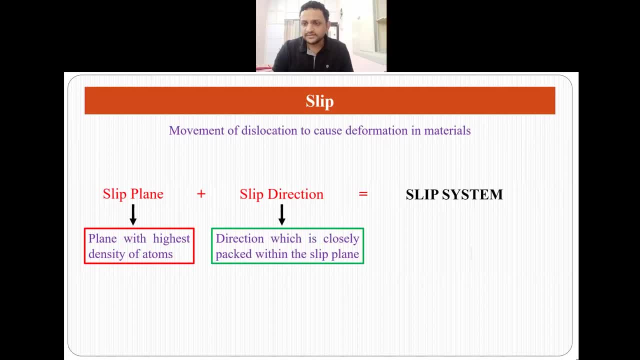 direction, which is closely packed within this slip plane, And the combination of slip plane and slip direction is what we call as slip systems. Now this slip occurs mostly in metallic materials. It is very, very hard to see slip process occurring in ceramics, composites or 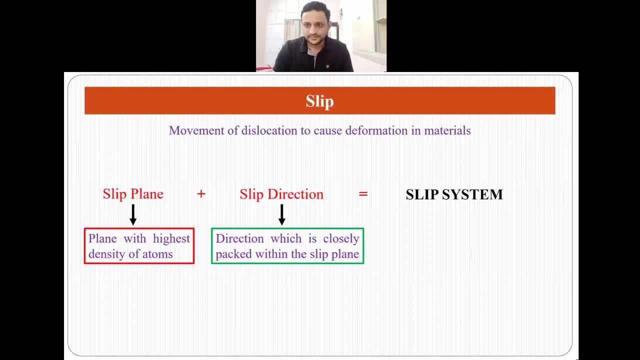 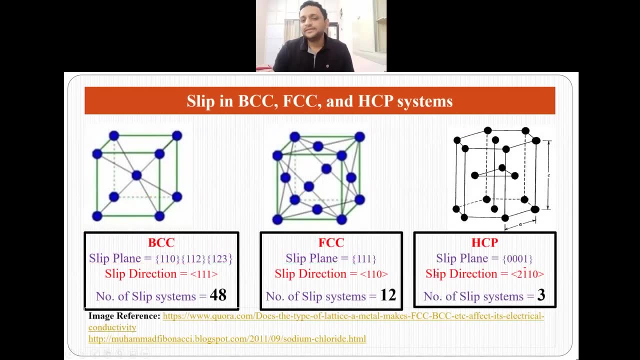 polymers or any other kind of materials. So mostly slip is seen in metallic materials And these metallic materials crystallize in either BCC crystal structure, FCC crystal structure or HCP crystal structure, which I discussed in my previous videos. Now these are the three diagrams of BCC, FCC and HCP crystal systems. The BCC has eight atoms and 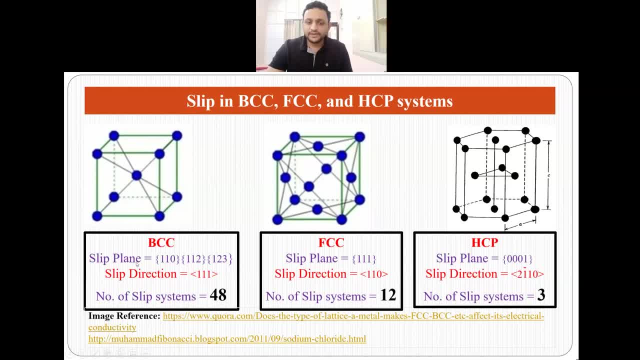 the corners and one atom at the center. Slip plane is 110, 112, 123.. These 110, 112, 123 are the family of slip planes, They are not only one slip plane. And slip direction is 111.. And if you? 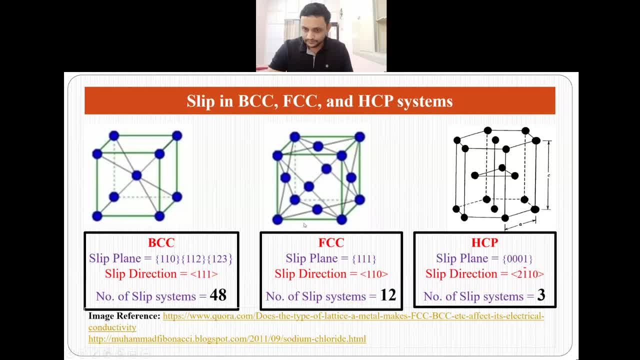 calculate. the total number of slip systems is 48.. In FCC we have eight atoms at the corners and six atoms at the faces. Here the slip plane is 111.. And slip direction is 110.. Total number of slip systems is 12.. In HCP we have 12 atoms at the 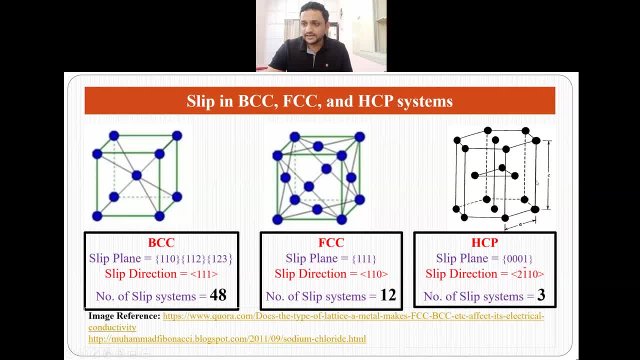 corners, two atoms at the faces and three atoms at the center, And the slip plane is 0001.. Slip direction is 21 bar 10.. And number of slip systems is 3.. Now you have seen that FCC materials have more ductile than BCC materials. And you may wonder why? Because BCC have a very high number. 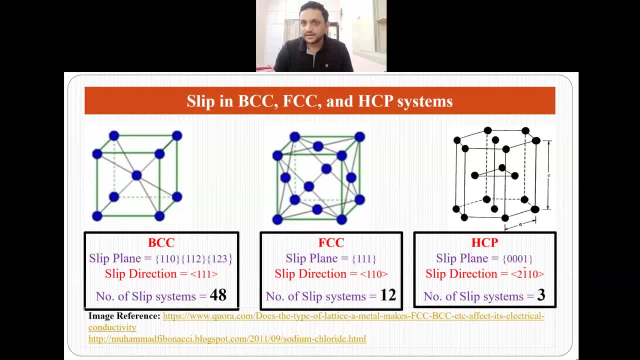 of slip systems. still, FCC materials are very ductile. So it may be confusing. The reason here is that the reason why the FCC materials are more ductile than BCC materials is because in FCC the atoms are more closely packed. If you see, the atomic packing fraction of BCC is 0.6.. 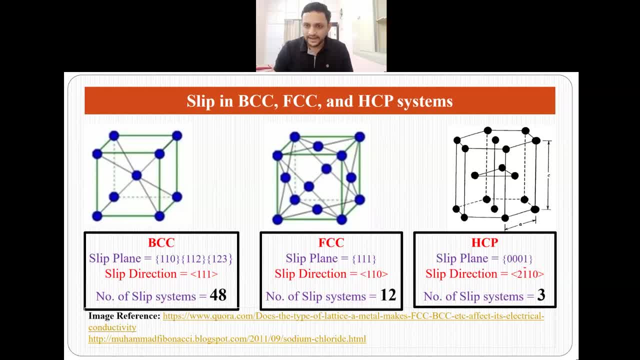 Or 68% of the volume is occupied by atoms. And if you see the atomic packing fraction of FCC, it is 70.74 or 74% of the volume is occupied by atoms. That is why FCC has more closely packed atoms And that is why deformation in FCC materials is much convenient and much. 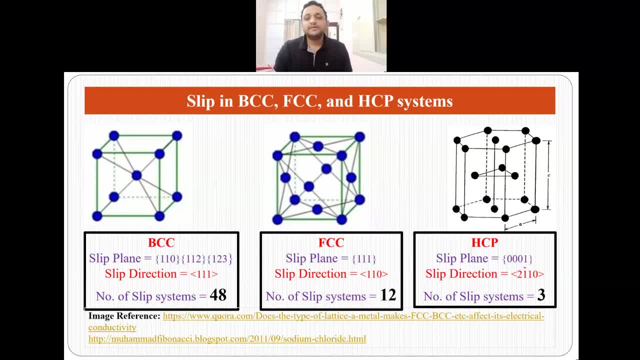 more easier than in BCC. That is why FCC materials tend to be more ductile than BCC materials, in spite of having lesser number of slip systems. So this is about slip in BCC, FCC and HCP systems. I hope you like my video and to watch more videos. 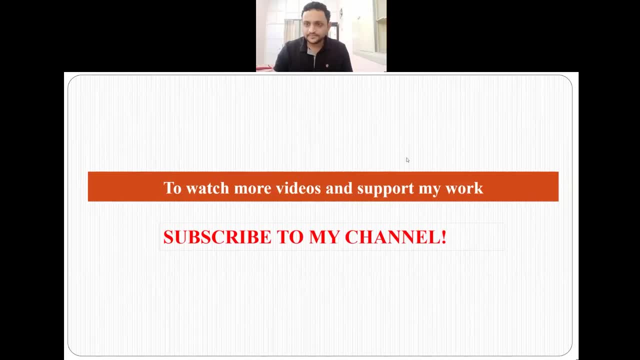 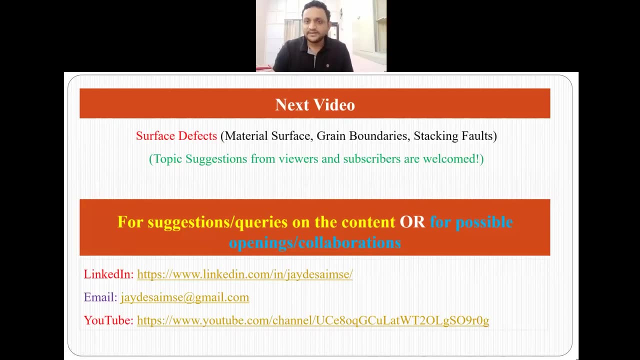 and support my work, please subscribe to my channel. And in the next video I will be talking about surface defects, That is, material surface, grain bound and so on. So let us start. Thank you for watching. In this video, I am going to tell you about surface defects, grain bound and stacking. 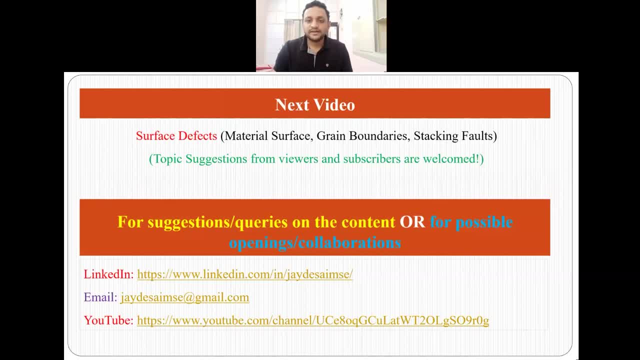 faults. Also, if you have a suggestion, if you are a viewer or subscriber and you have a suggestion, please comment in the video below, in the video so that I can make videos on that, And for suggestions, queries on the content or for possible openings and collaborations. 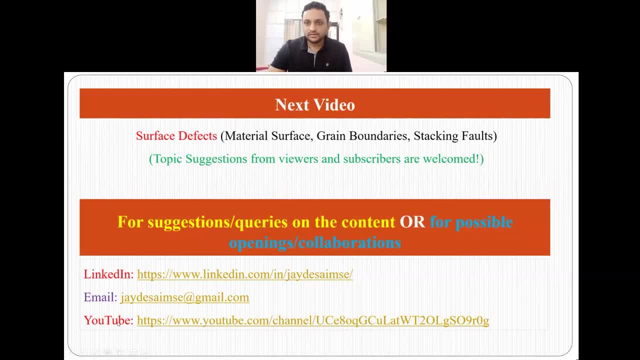 you can reach out to me via LinkedIn email or by commenting in the YouTube video. Thank you, Thank you.